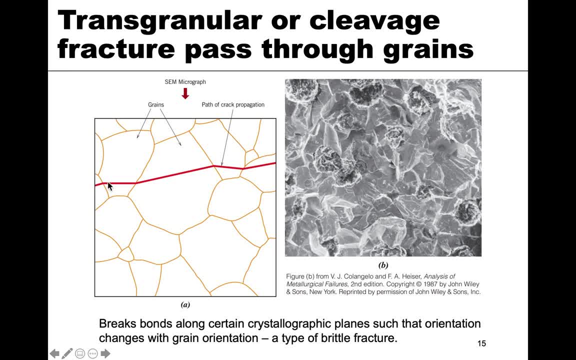 this is the path of the crack propagation. And this is the path of the crack propagation, This is the splitting line. So this is one new surface and this is one new part up here. That's where the bonds broke And when you look at this you'll have an appearance kind of like you know. 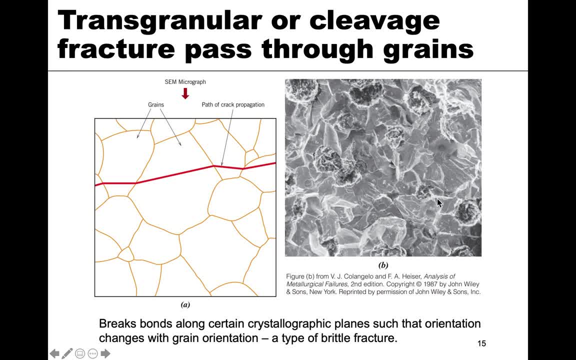 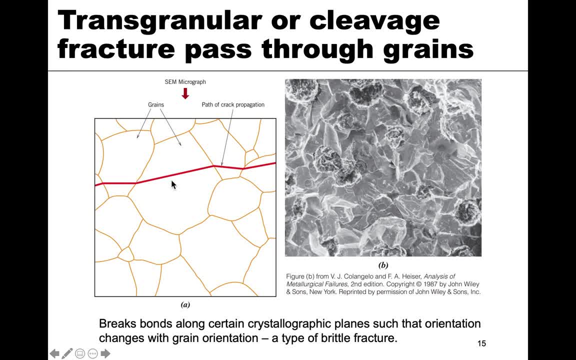 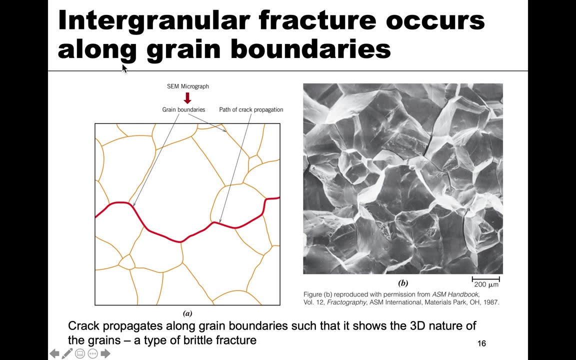 across a number of parts. So that's one type. And this, again, this is from a polycrystalline material. where you see, where you see this, You can also have it. the opposite occur: intergranular fracture. This is when it occurs along or through grain boundaries, right? So here? 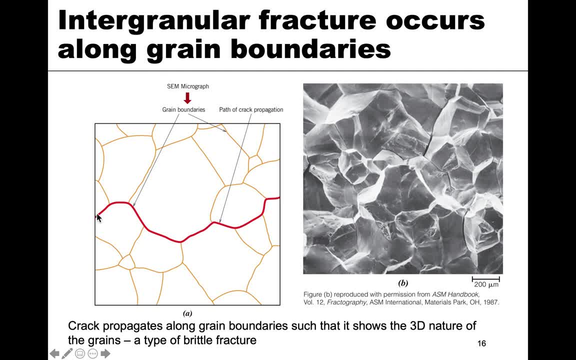 you can see the same kind of general microstructure, But here the red line, which is the path of crack propagation, is the path of the crack propagation. And this is the path of the crack propagation. It's basically along the grain boundaries, So it doesn't go through the grains, So it's 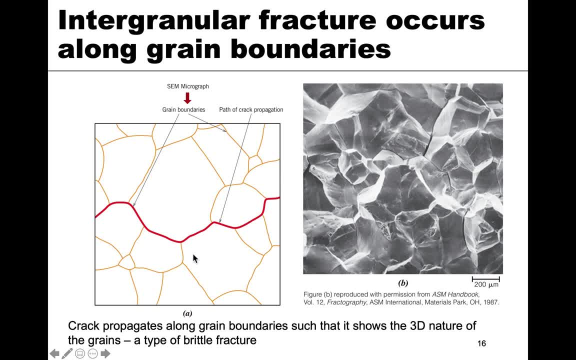 intergranular. And so here, when you look at this, the result of these new surfaces, and this is what you can see here- you see that it's a very smooth surface And you see basically what looks like grains. So you know, you're basically looking at the surface of the grain, And so you can see that. 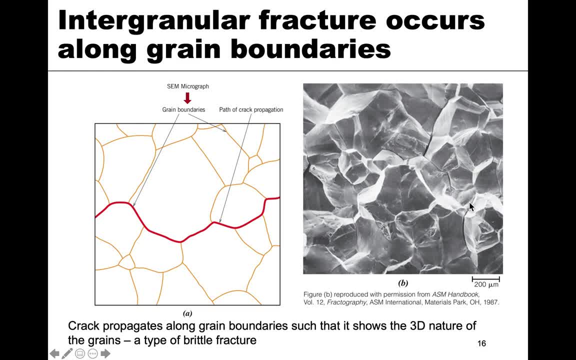 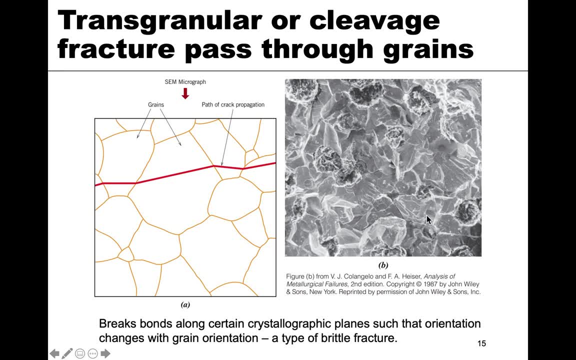 kind of shape And it's going to follow that structure. So it follows the grain structure. So it's a little bit different than here, where it's a little bit rougher. The actual surface is rougher and it doesn't necessarily follow grain boundaries, So it's more. it still has some. 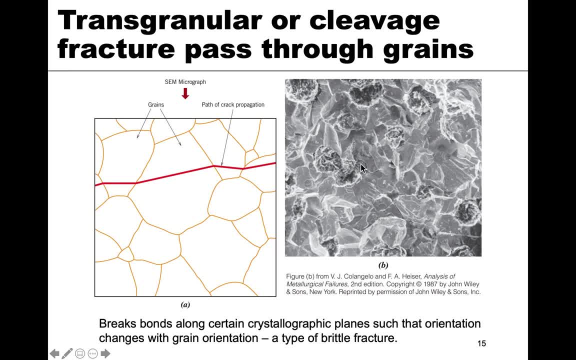 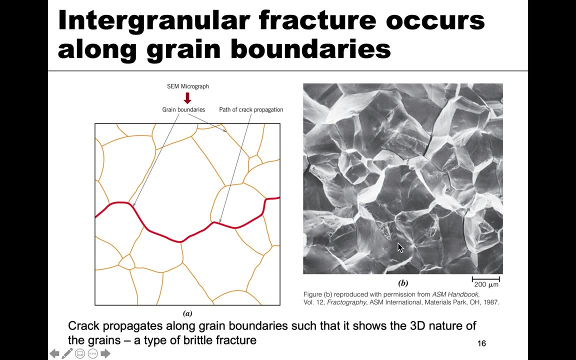 texture to it, but it's not following the grain structure as much as it's following the kind of path of crack propagation. So there's some more texture on the surface as well. So that's kind of the main difference, And so you can see the grain structure. And so you can see the grain structure. 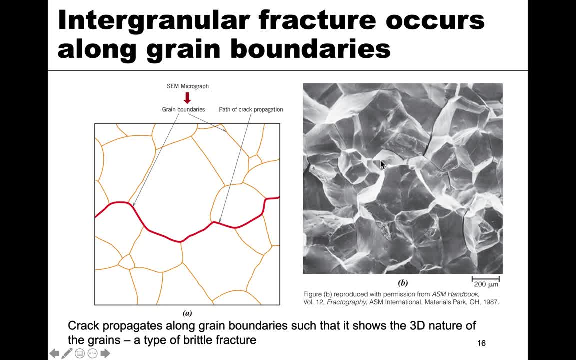 and you can kind of see the 3D nature, which is why SEM is good. because of that depth of field, we can see this type And again, this is a type of brittle fracture that occurs All right. so let's look at. 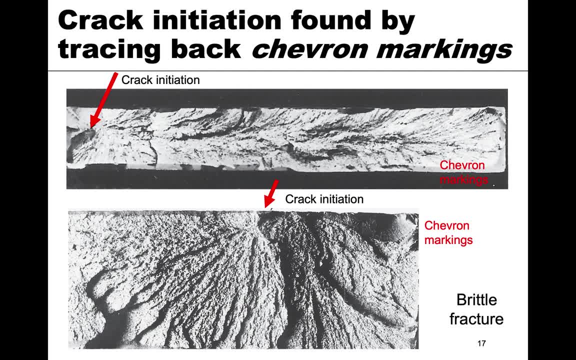 some other kind of fracture surfaces and what we can get out of them. So this is a test sample. I believe this is from a impact sample, which we'll talk about later, But in essence you can kind of see that there are different lines and patterns on the sample And this actually can be used to. 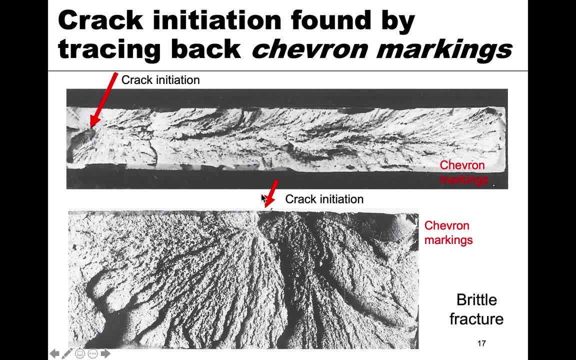 determine where crack initiation comes from. So here, all these kind of lines, if you can kind of follow them back, kind of lead to this point And it's a little bit more clear here, because all of these lines we call them chevron marks or river marks. sometimes you can see all of these. 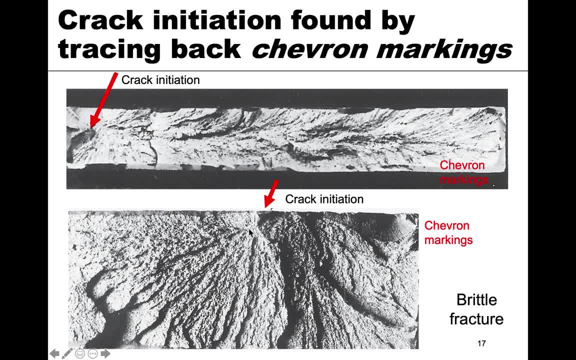 chevron markings kind of point back to a single point here. So basically it's here or it's here or right here on this surface, And so chevron markings can tell you where crack initiation occurs, And that's important right. we can kind of identify it back to a feature on the surface or at. 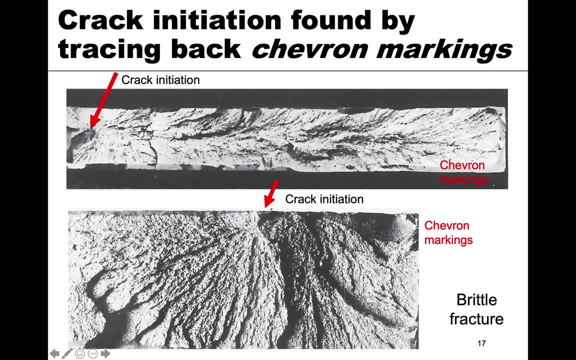 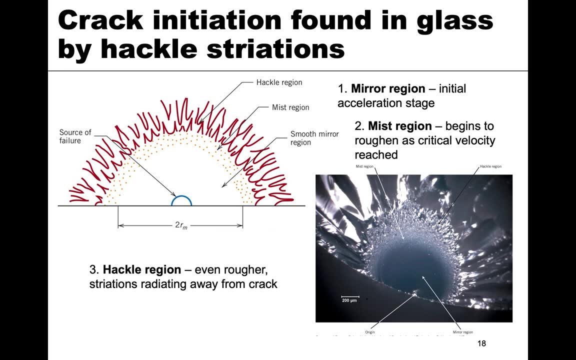 this notch that we see, And so that's helpful for determining the initiation and maybe what caused it in your kind of postmortem analysis. We can do the same thing with glass, So with amorphous materials like inorganic glasses or polymeric glasses, those fracture surfaces tend to have a very unique fracture, So it's still 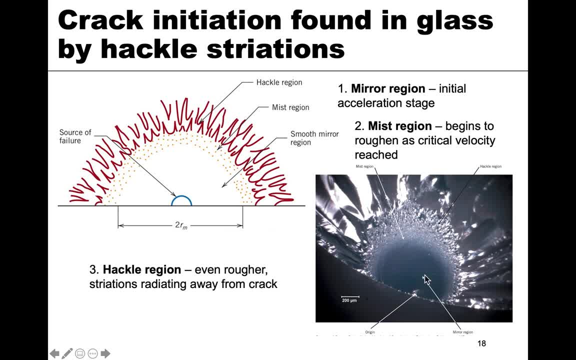 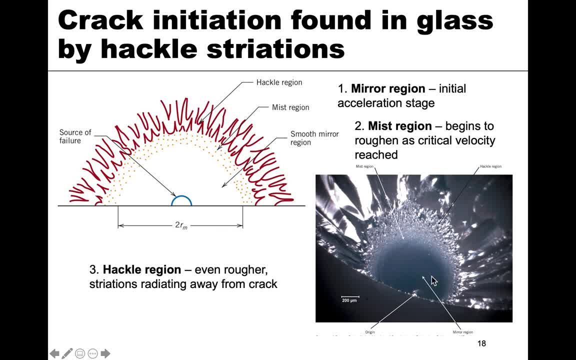 the surface. But then we see this kind of smooth region. This is known as the mirror region. It's where the crack initiation initially accelerates. So it's basically smooth in that region because it's accelerating up. And then you get to a certain point where it stops being a smooth and we 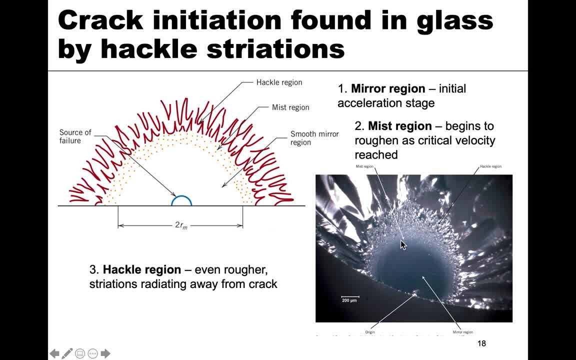 call that the missed region, because it kind of looks like mist and kind of spots And it looks a little hazy. And then you see an expression of snow or something that it's called a kind of, and so that's where it begins to roughen because it stopped accelerating and you 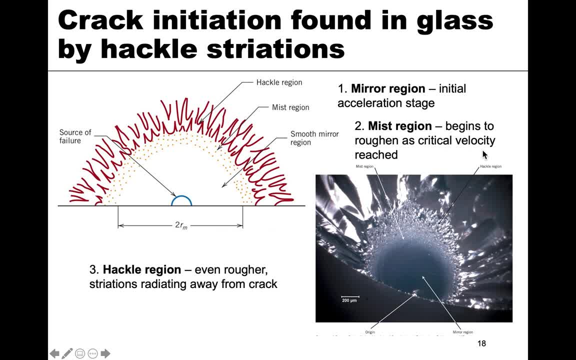 reach a critical velocity of the acceleration because it's brittle fracture and so it happens really quickly, and so that's where you've basically reached that acceleration, and so it becomes more roughened and then, a little outside of that, you start to see the hackle region, and this is the even. 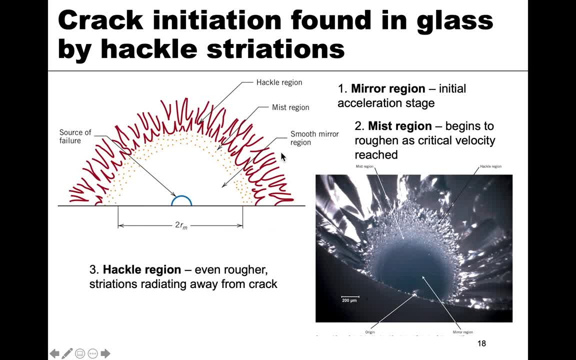 rougher and then this is where you start to see those striations which point back to the initiation. so this can be quite large and you can actually see quite a bit of the striation here. so that's the hackle region. it's even rougher and it has those striations leading back or radiating away from the 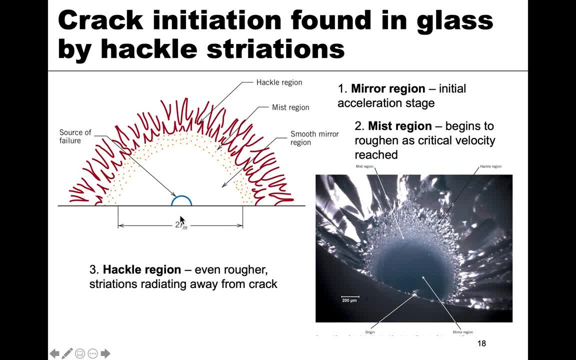 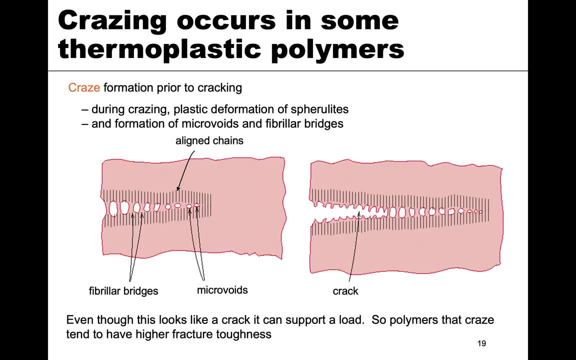 crack and so that kind of initially points you back to where the source of the failure may have been. so that's kind of an amorphous glass materials, so no grain structure, so not like the inner or the inner versus transgranular. another phenomenon called crazing. this is something that 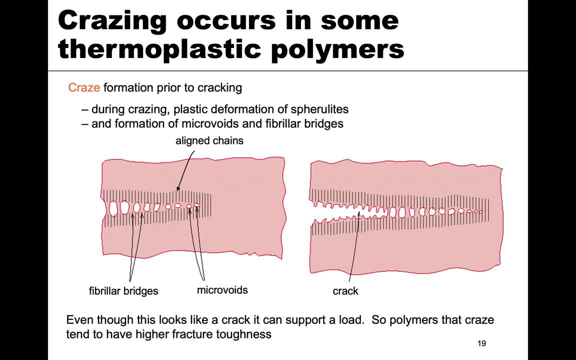 happens in a lot of thermoplastic polymers. so we're going to talk about polymers here in the next chapter, but for now I just kind of want to point you to the, the fracture that can occur. so again, it's, it's crazy and basically what? 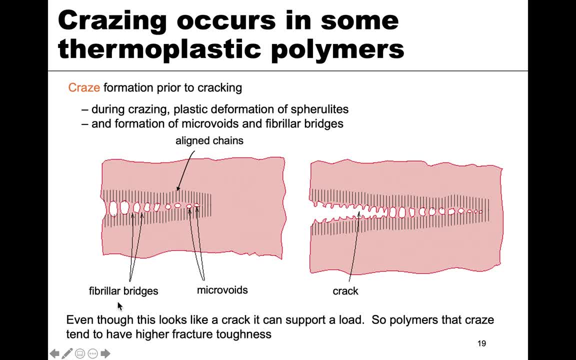 happens is, with this polymer you have a linear kind of strand structure so that you have all these chains of polymers and they're all aligned and the vertical direction, and so when it's being extended and you see that it's trying to open up this region, 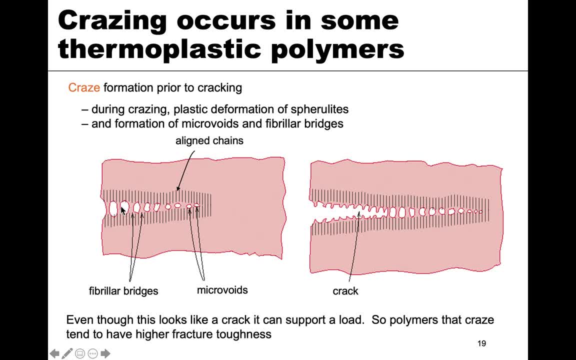 you start to see those voids occur, and they occur kind of between, as individual strands are breaking, so the bridges of these fibers are breaking in those portions and connected elsewhere and so then eventually at some point these are going to kind of connect up. it's going to have this sort of jagged tooth phenomenon and that.